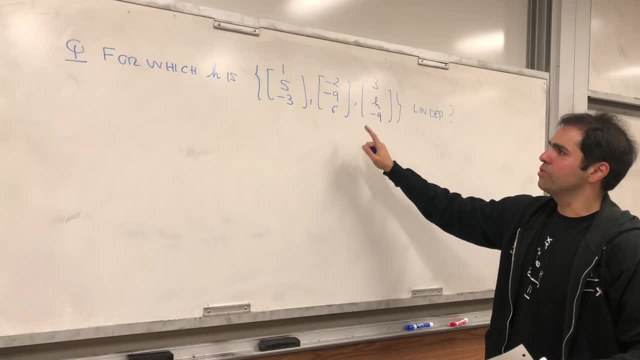 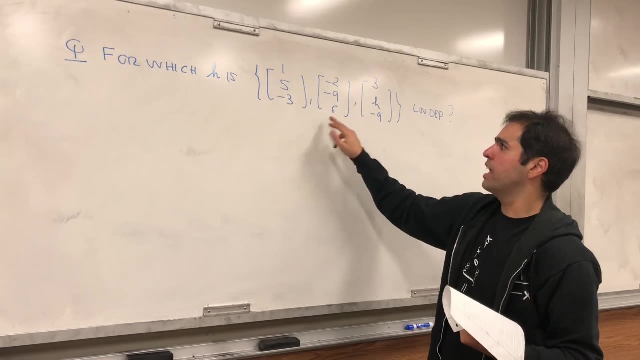 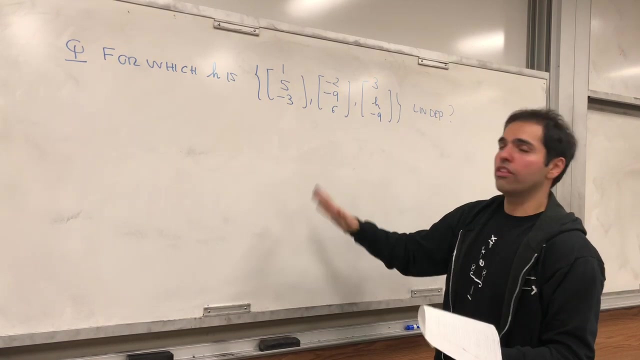 It means there's some relationship between those two, three vectors. and be careful, relationship doesn't mean that the first vector can be written in terms of the other two. It could really mean one of those vectors can be written in terms of the others And to write this more compactly is the following: Are 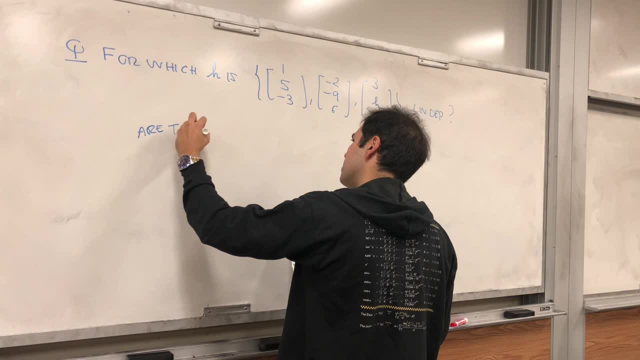 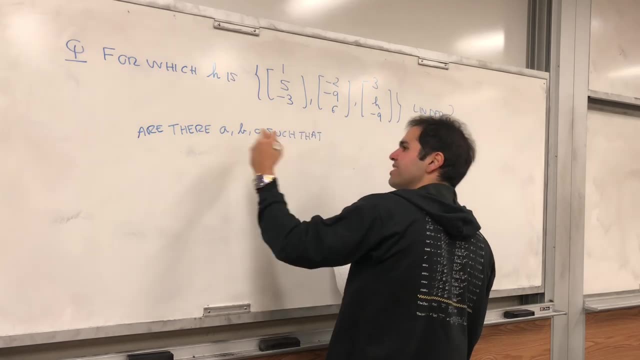 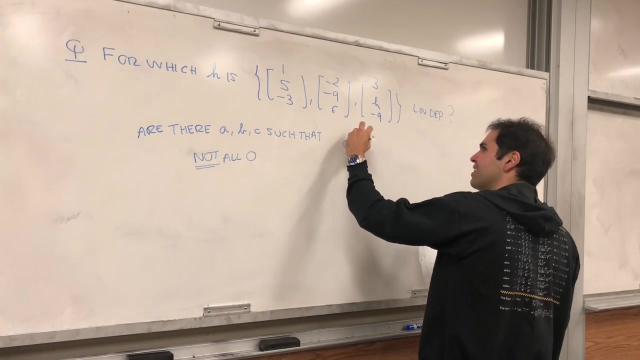 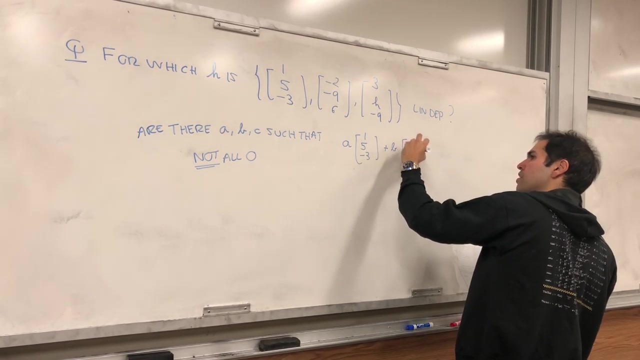 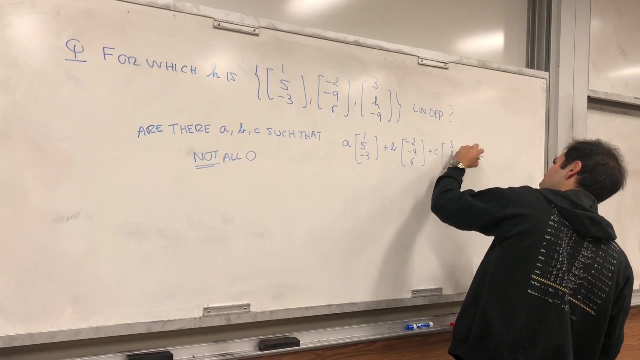 there a, b, c, such that so a, b, c, not all zero, so very important- such that a times the first vector plus b times the second vector and c times the third vector equals to the zero vector. So it's a compact way of writing. there's some relationship between 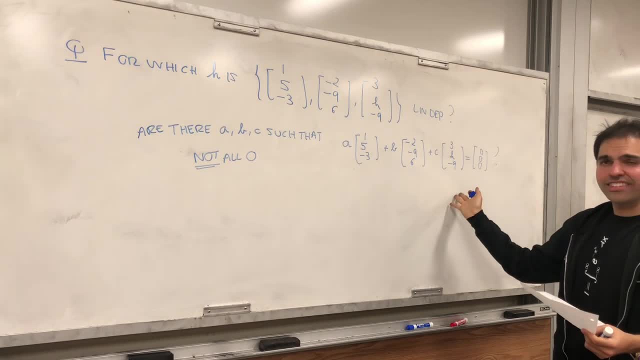 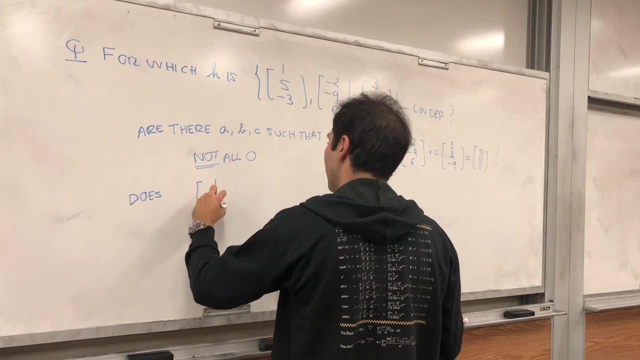 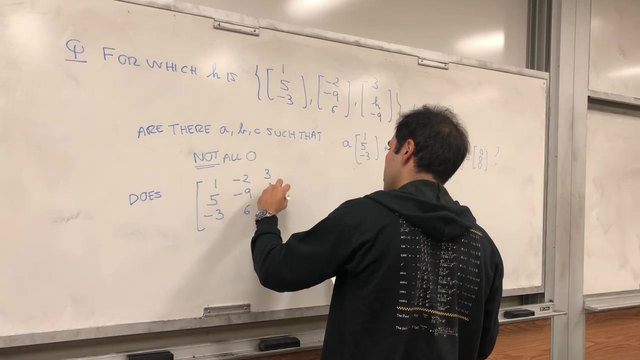 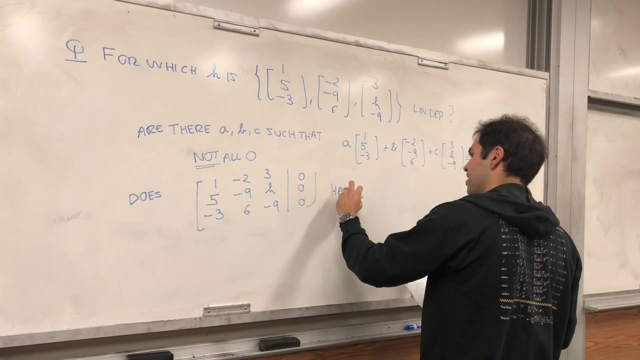 the vectors And notice in terms of systems. all this means is simply: does the following system: 1, 5, minus 3, minus 2, minus 9, 6, and 3, H minus 9, and 0, 0, 0 have- and I'll put some space, a something solution? 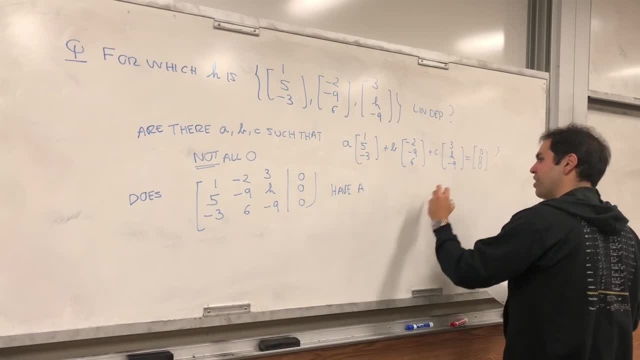 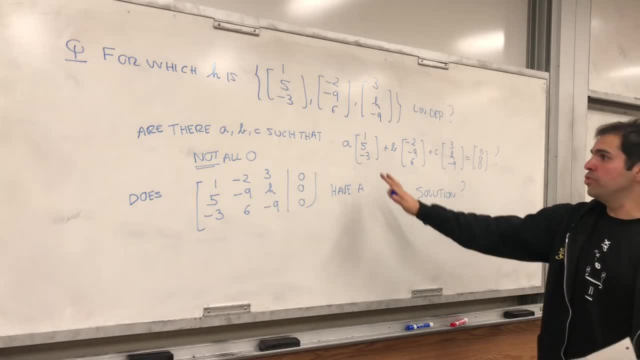 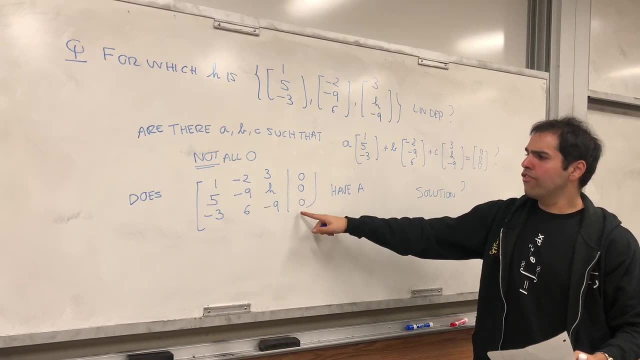 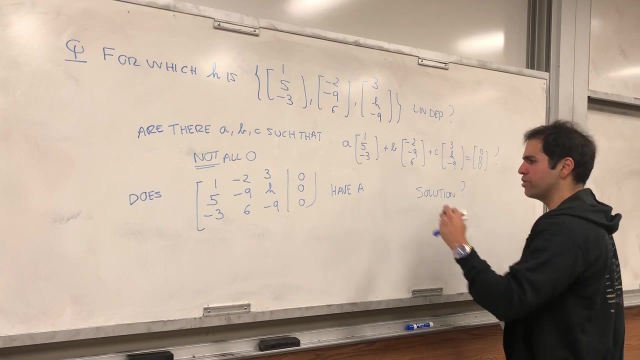 This system always has one solution, because you can always let a, b and c be zero, and that's fine. So things of the form a, x equals to zero always has a solution. The question is, really, does this have a non-zero solution Now? 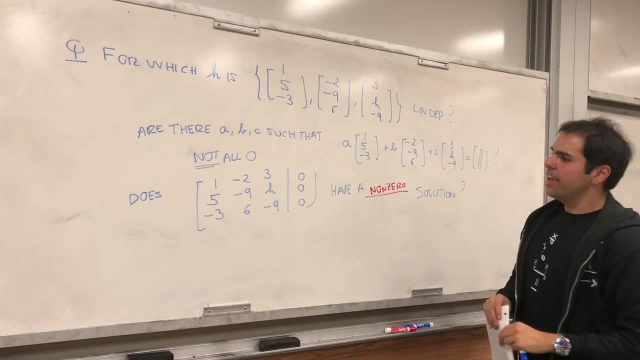 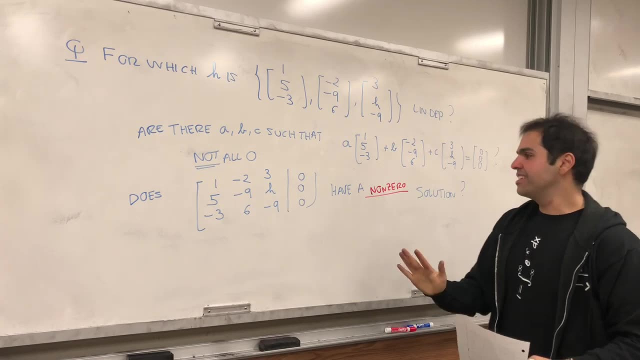 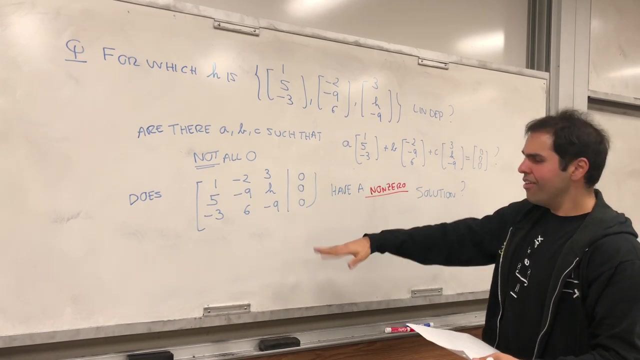 Now what do I want to say? Again, here is a stupid way of doing it and a smart way. So the stupid way is actually solving the system. We don't have to do that, We just need to figure out if it has a non-zero solution. So let's take this and 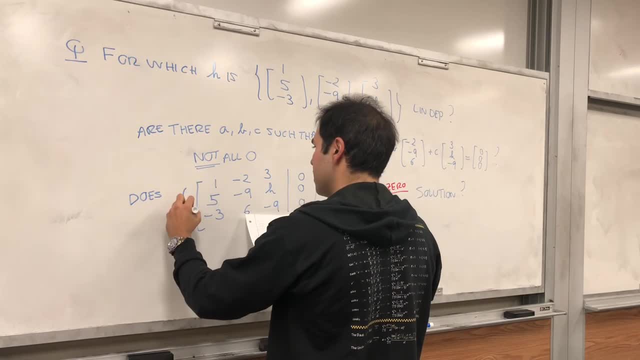 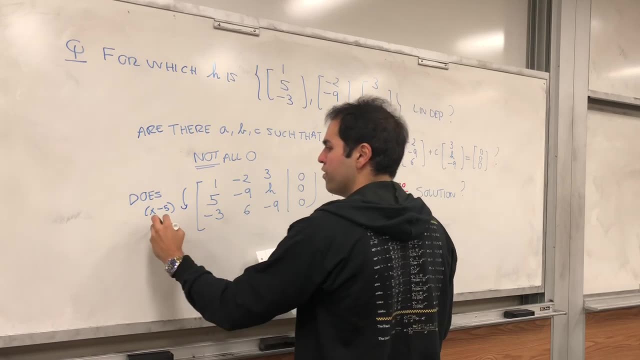 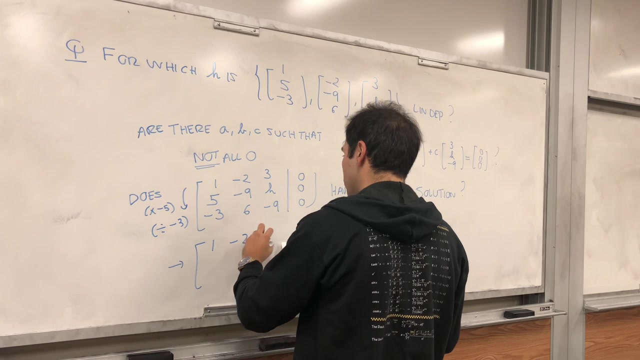 row reduce. So let's, for example, add minus 5 times. So, in other words, let's subtract the first row from the second row and also here we have a simplification- can factor out minus three if you want, and you get 1 minus 2. 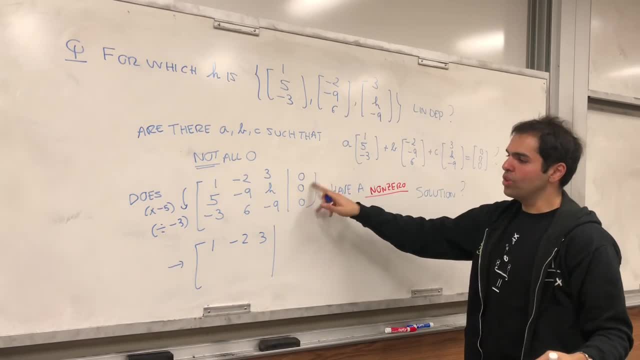 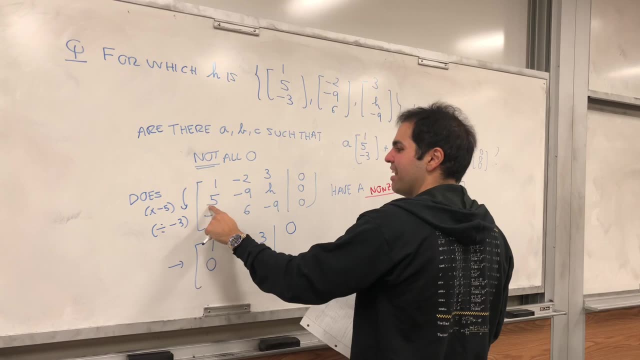 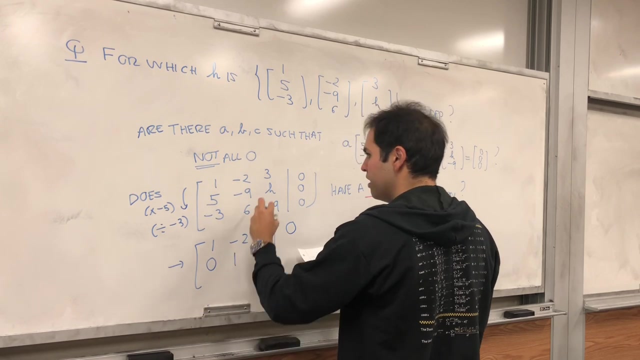 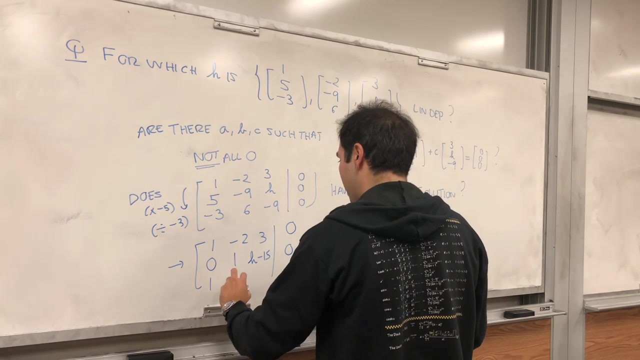 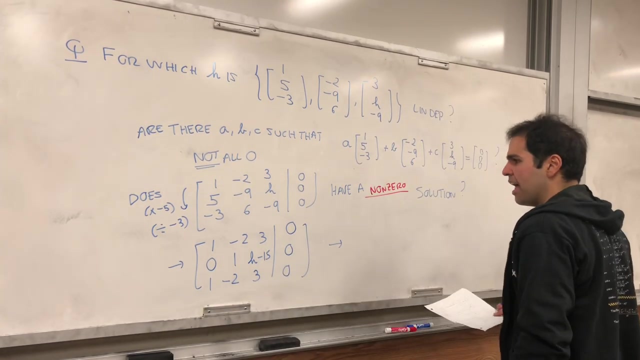 3, and notice, ax equals to 0 is so easy. you don't have to worry about the right hand side. that's why they're happier systems. so, and 5 minus 5 is 0, 9 plus 10 is 1, and then H minus 50 and 0, and then this becomes 1 minus 2, 3 and 0, and then 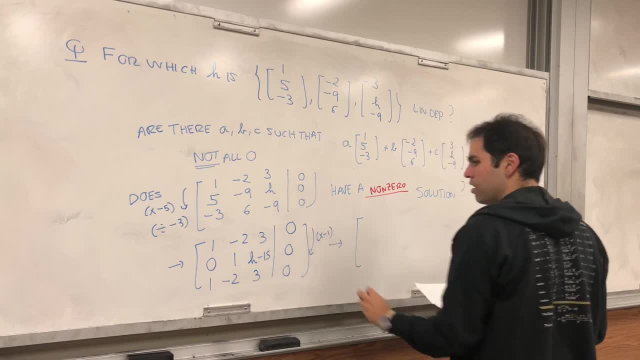 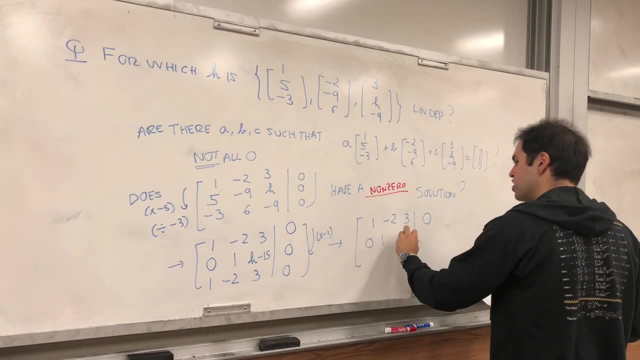 one thing you can do: you can subtract and we can do 1 minus 2, 3, 0, and then 0, 1 H minus 50 zero, and then, well, in fact it was just 0, so 0, 0, 0, 0. 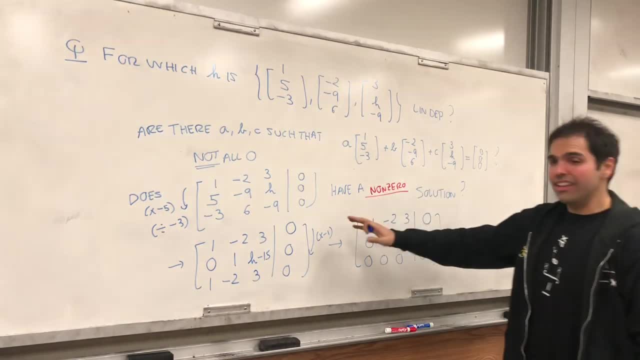 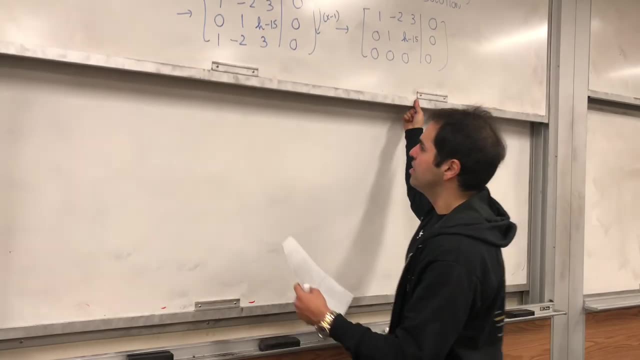 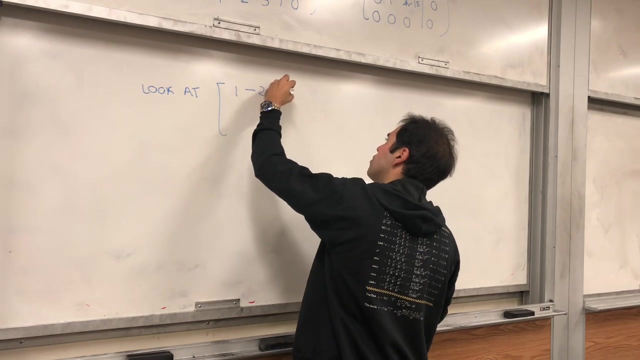 yes, very okay. now it turns out, I realized we didn't even have to put the 0 0 0. let's just work with this coefficient matrix. so just look at 1 minus 2, 3 0, 1 H minus 50 and then 0 0 0. 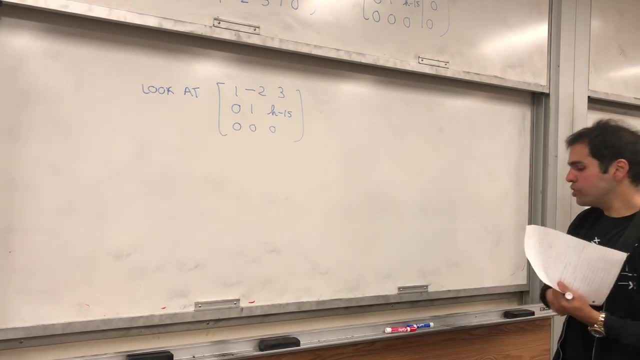 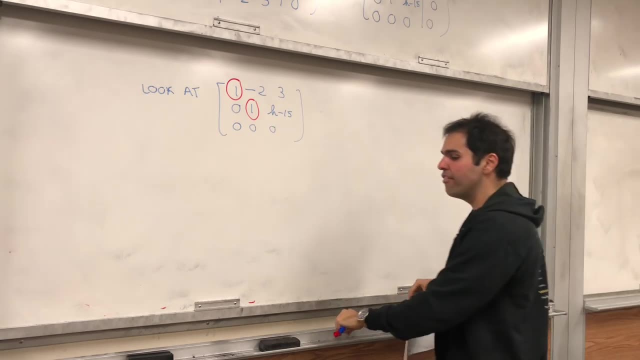 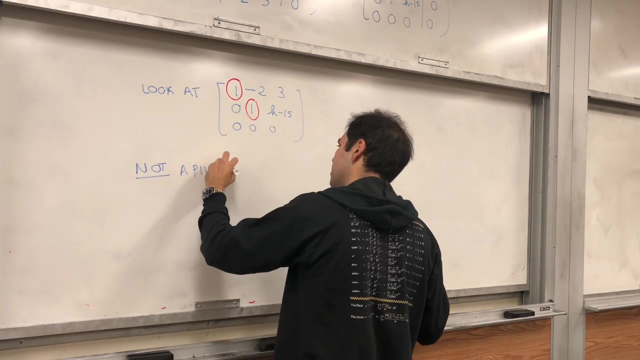 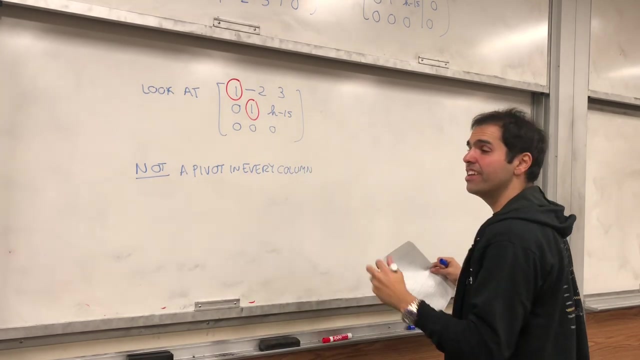 0- zero. What are the pivots? There are two pivots here And in particular we don't have a pivot in every column, So not a pivot in every column. And it turns out, if there's not a pivot in every column, technically it means that the columns 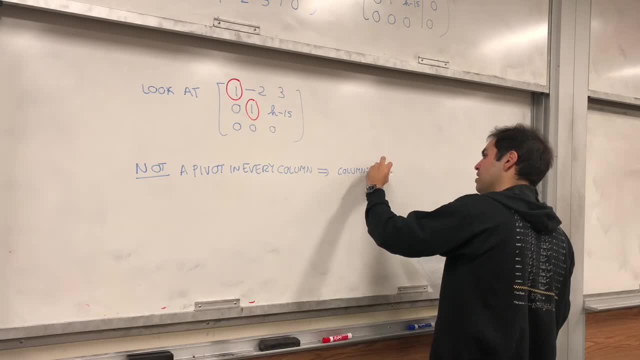 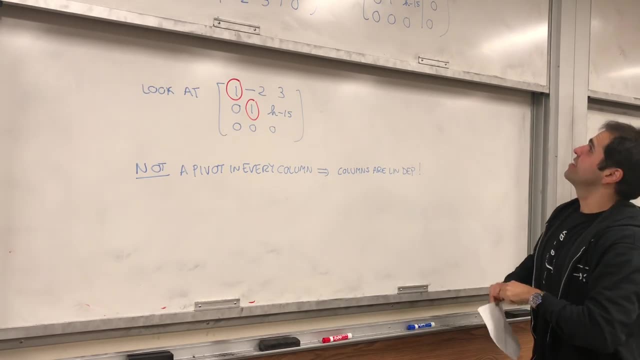 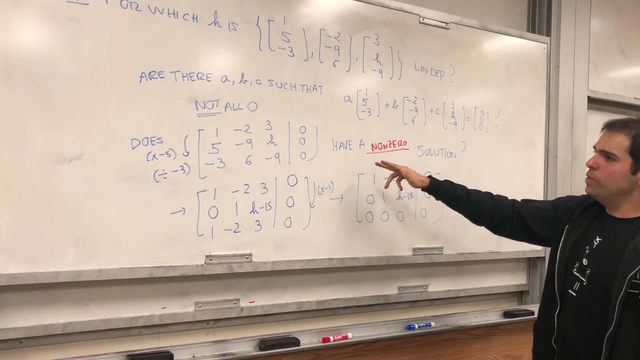 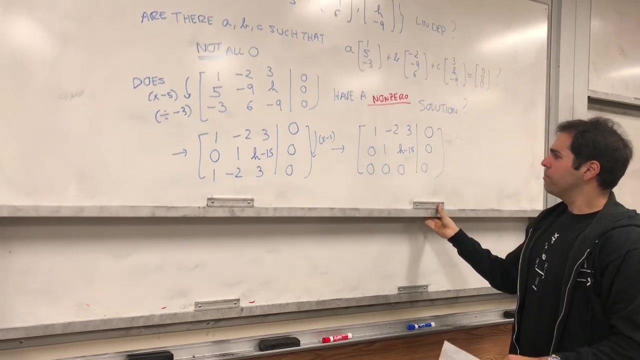 are linearly dependent. Why is that? Because look at this picture. if I could look at this matrix again. As I said, we don't need to figure out what the solution is, We just need to know if it has a non-zero solution. So, in particular, 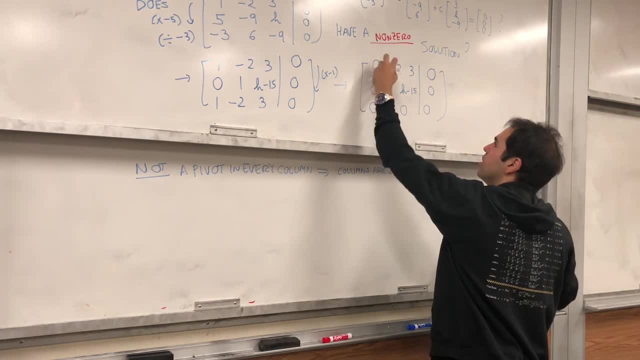 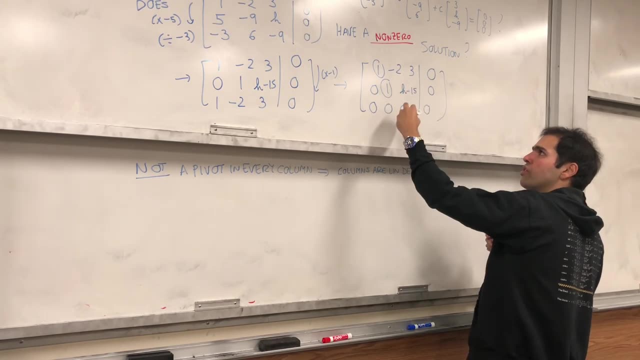 because of thearc trading zeg the included j to all the PRIDOMs in A. one of their problems is that non-zero solutions don't affect only the matrix A, f or n, etc. And the pivots are here. Interestingly, no matter what the value of h is this third column? 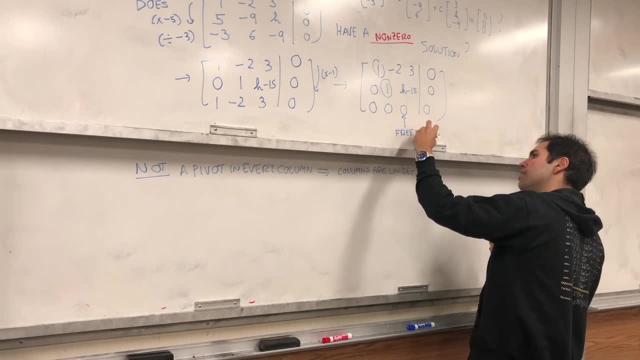 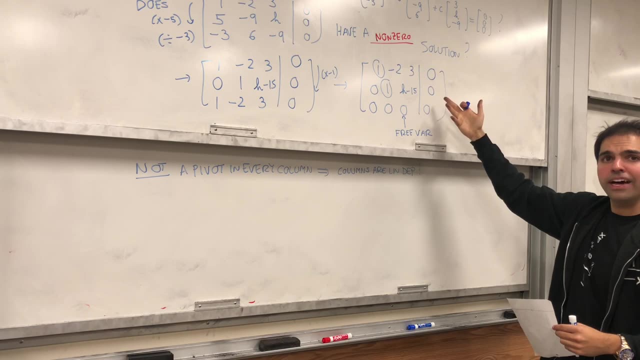 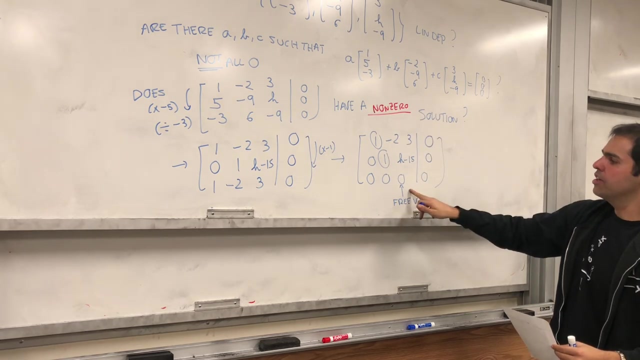 will always be a free variable column, And because this system will have a free variable, it automatically means it has infinitely many solutions, Because it has at least one solution, the zero vector. so it either has one solution or infinitely many, But because they're free, 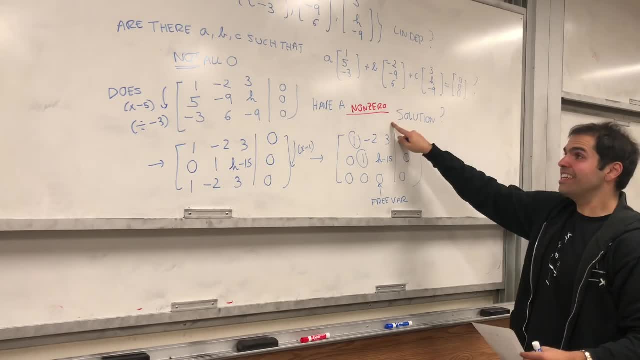 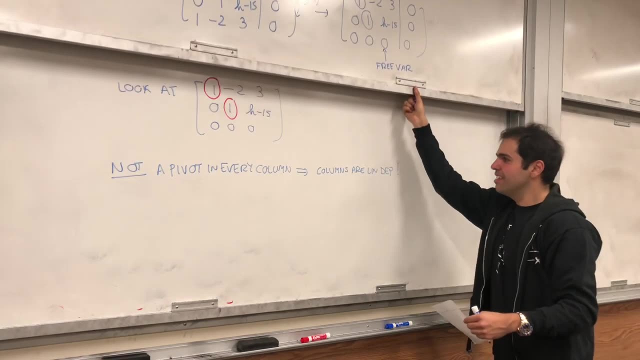 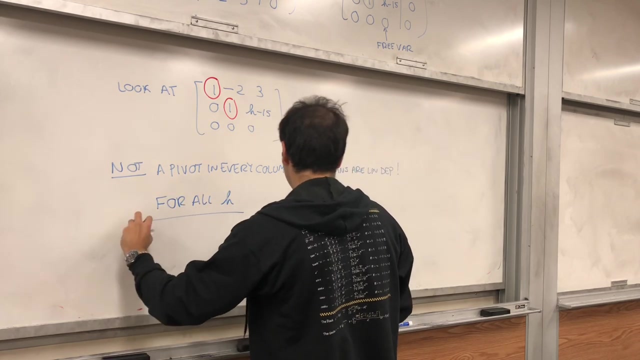 variables, it must have infinitely many solutions. In particular, it must have a non-zero solution, And this means that the vectors are linearly dependent. So the answer is then: for all h- Interestingly for all h, this has a solution. I mean for all h, it has a solution. but 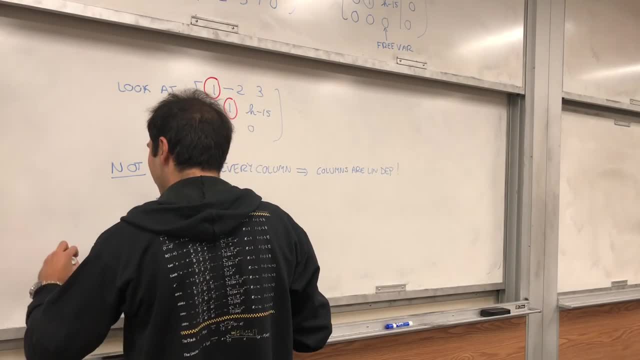 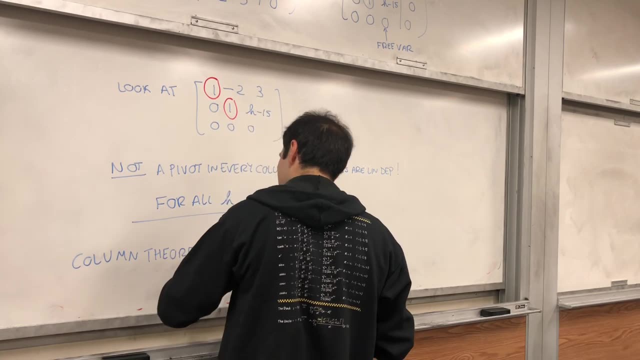 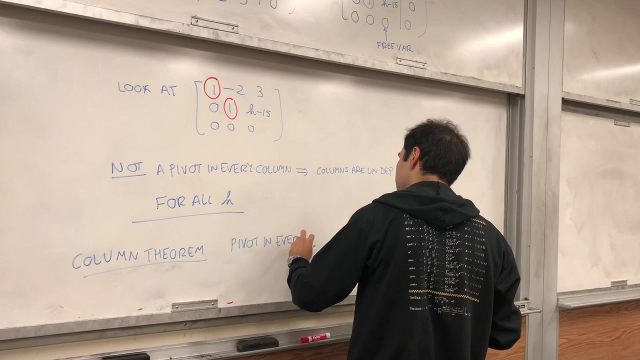 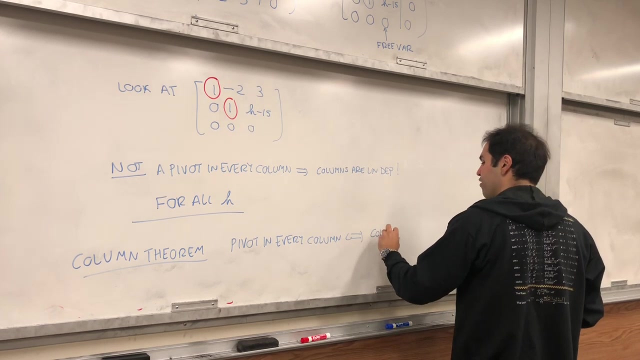 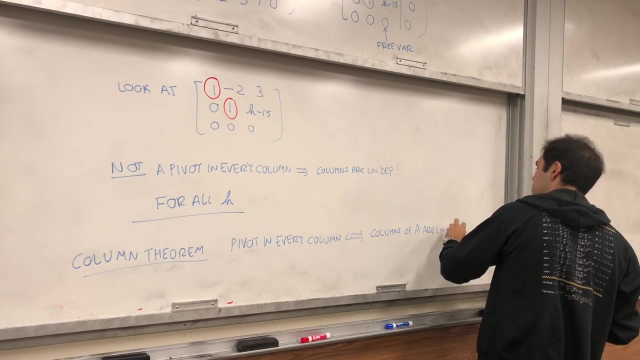 this is linearly dependent, and let me sort of summarize that by what's called the column theorem. so if there's a pivot in every column of the coefficient matrix, that's the same implies also that columns are a, of a are linearly independent. that's because if there's a pivot in every column, there are no free. 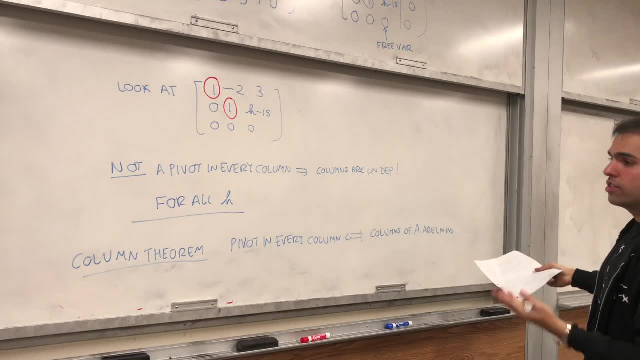 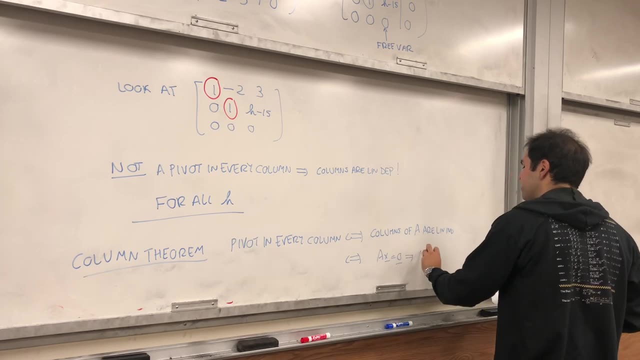 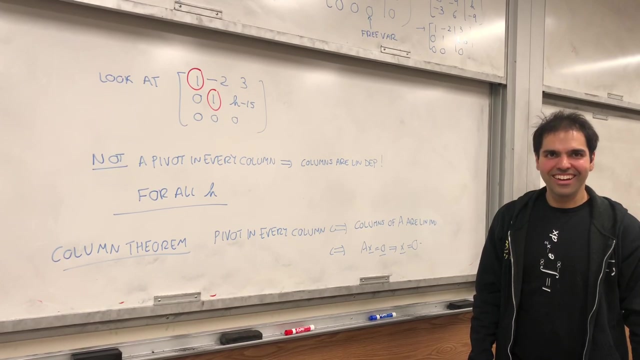 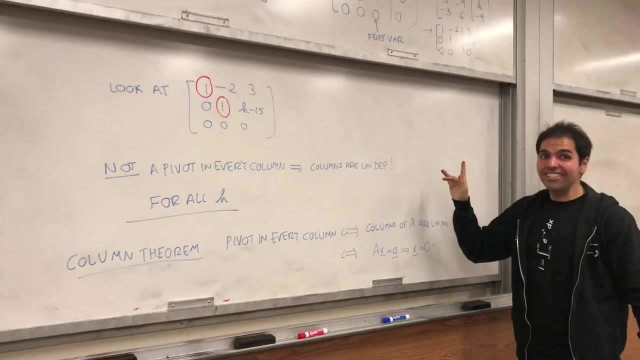 variables. so ax equals to zero must have just the trivial solution. and by what I just said, it also means that ax equals to zero implies x equals to zero. wait, Payan, you stress seriously for OH that this right here will be linearly dependent. no, it's very surprising, but let me show you. so what if H is one, for example, like: 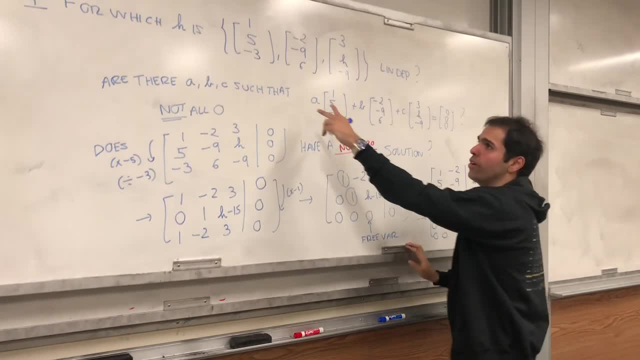 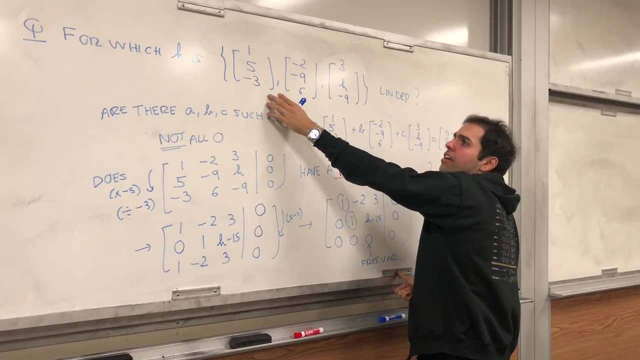 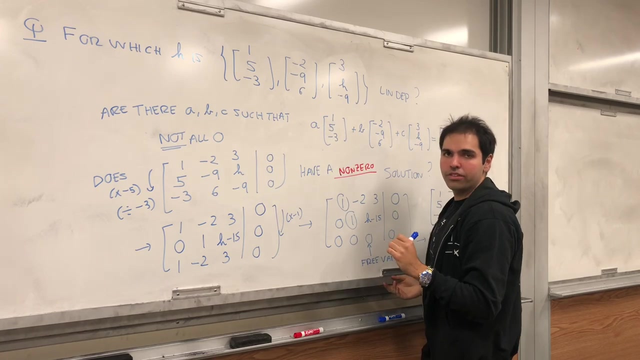 okay, let me show you. so the question is, first of all, those two vectors. they're not- well, they're not multiples of each other, they're not already linearly independent. so the question is really, is this vector in the span of the other two? yeah, okay, let's do it with the case. H equals to one. yeah, it gives you a very. 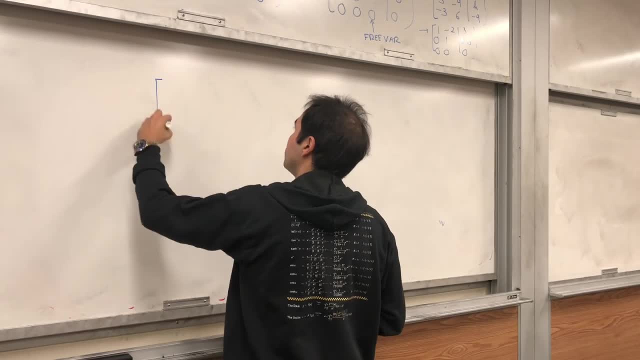 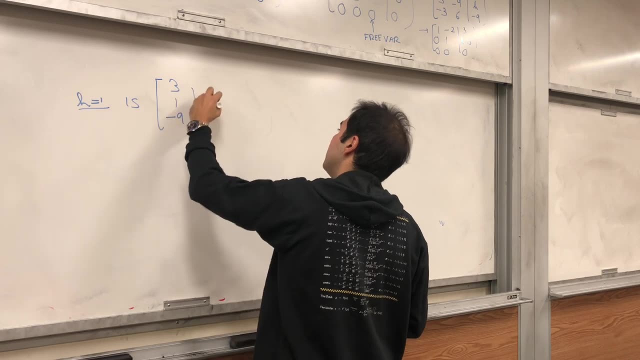 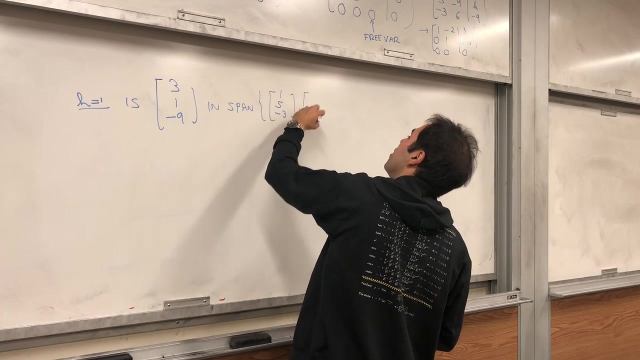 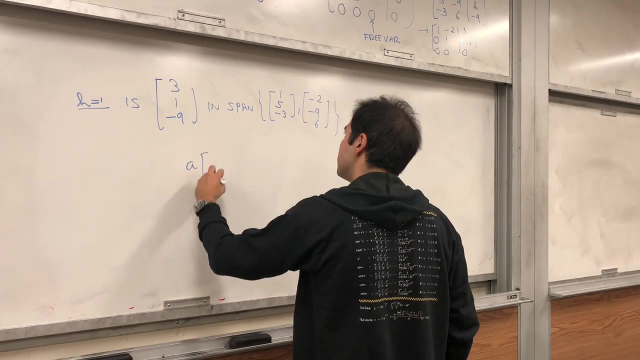 surprising answer by the question is: let's do it with H equals to one, is the vector three one minus nine in the span of the other two vectors, one five minus three and minus two minus nine, six, and in fact let's try to find a and b such that a times one five. 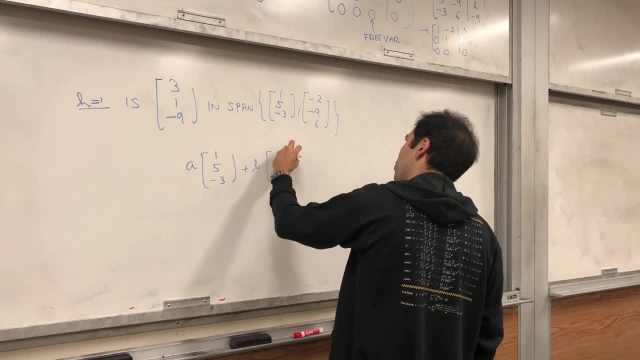 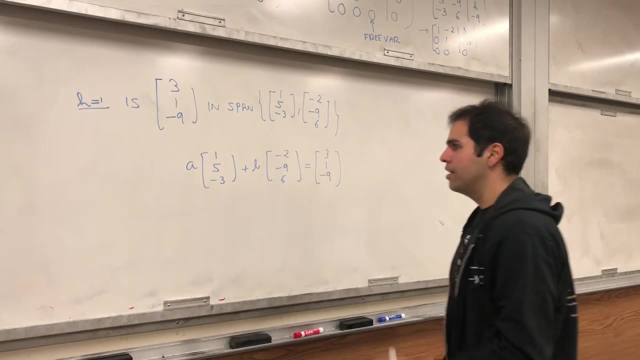 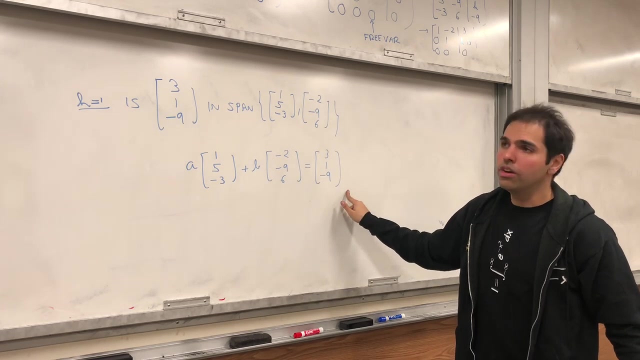 minus three plus b times minus two minus nine, six equals three. one minus nine. one little remark. so technically the question is: are there a and b? such as this is true, yeah, so technically we don't have to solve the system, we just need to check if there's a pivot in. 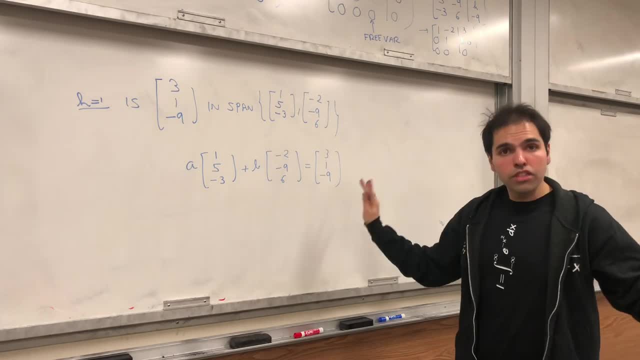 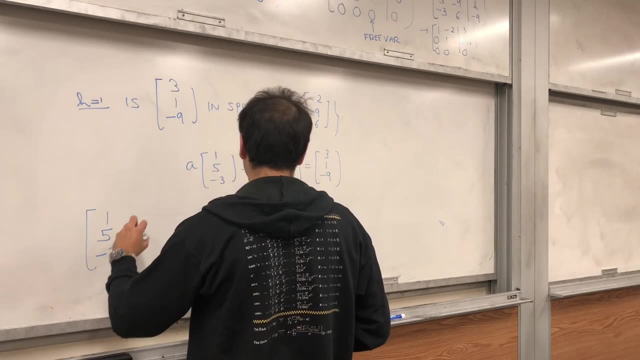 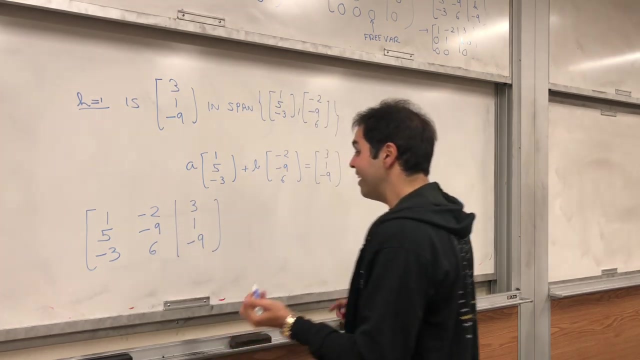 every row of this matrix. but just for sake of completeness, let's try to solve it. so if we do one, five minus three, and then minus 2 minus 9, 6 and then 3, 1 minus 9, the good thing is we've already done. 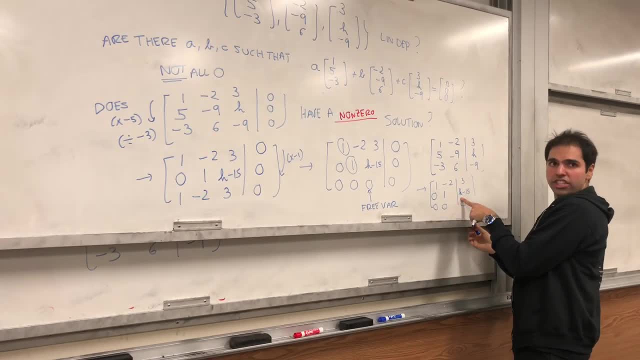 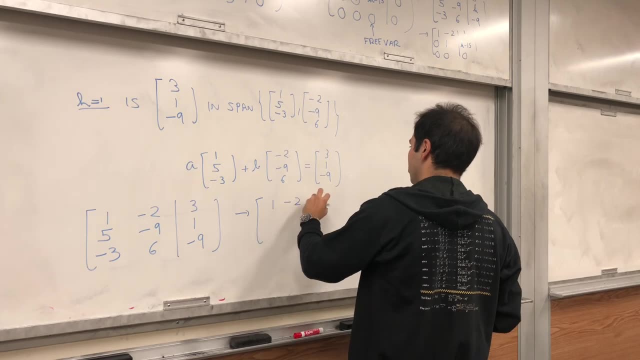 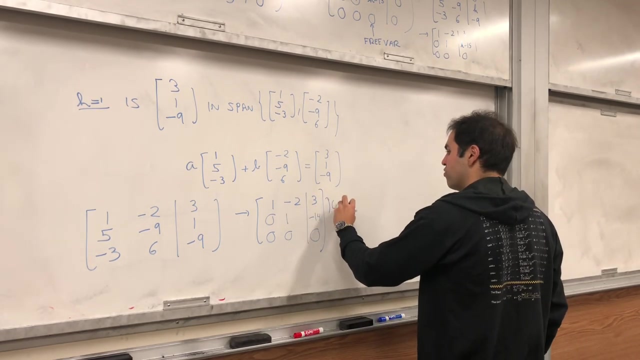 that. so we already had this, but with H equals 1. okay, so this gives you 1 minus 2, 3 on minus 2, 3 and then 0, 1 minus 14, because H is 1. yes, okay, and let's continue. so let's do reduced row echelon form, so times minus 2, and it gives you 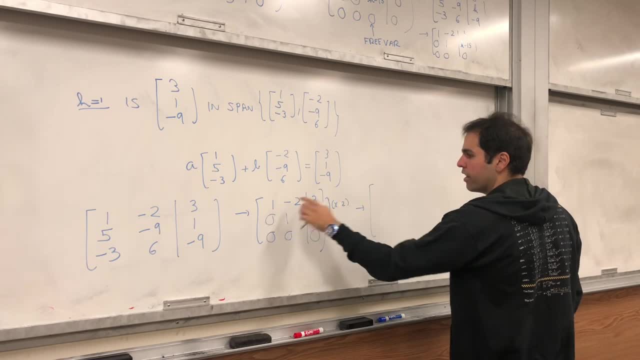 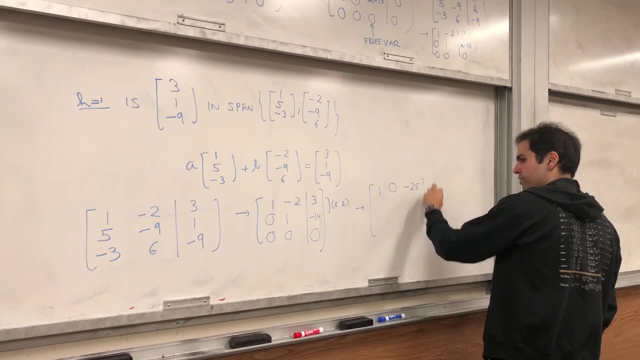 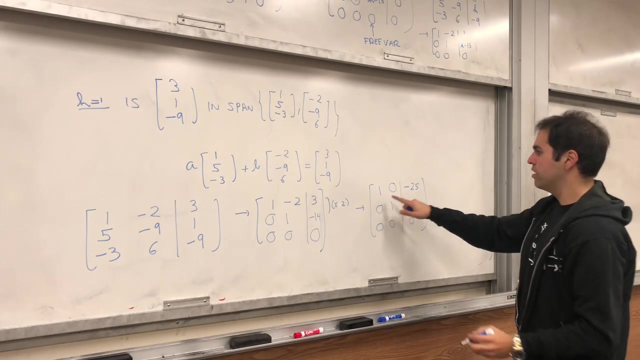 so I guess times 2 times 2, and then 1: 0 and then so minus 28 plus 3, that's minus 25, minus 14 and 0 0, 0. so it turns out back, substituting: a is minus 25 and B is. 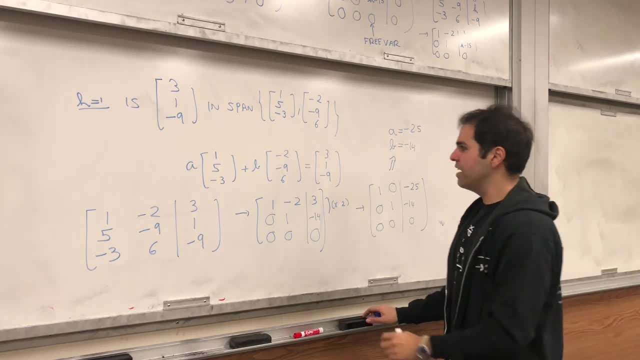 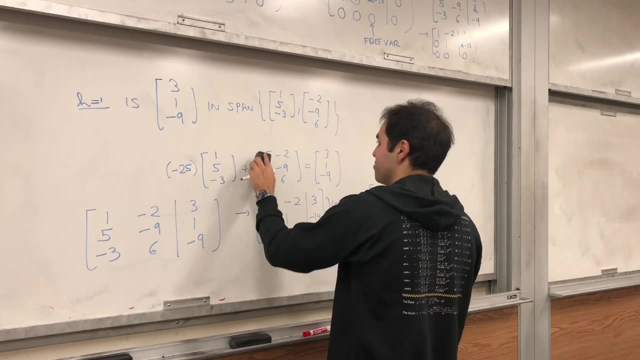 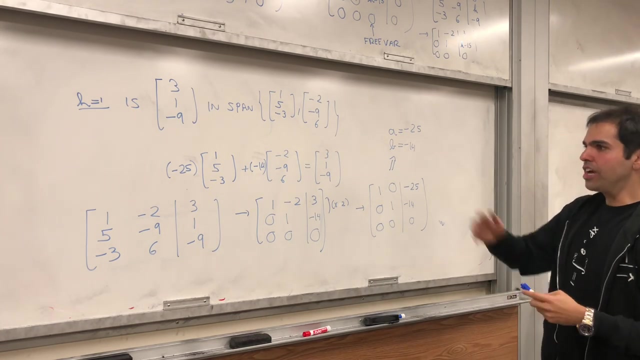 minus 14. so 3, 1 minus 9 is minus 25 times this vector plus minus 14. I think it's very impressive. who would have guessed that? yeah, you can check that this is correct. and, by the way, is that the only pair of a and B that will make?